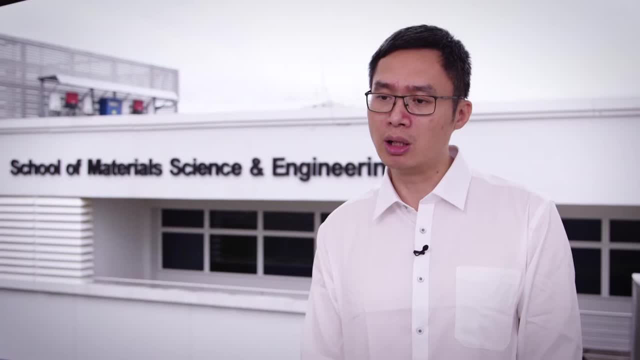 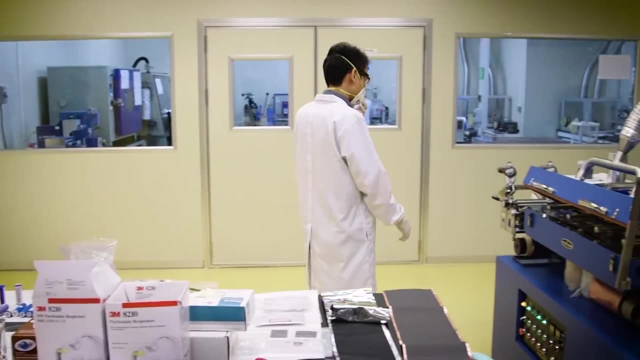 collaborative colleagues. They can help you with your research. They can help you with your research. They can help us to design materials modeling simulation. In the end, we can really evaluate the performance of materials. ARIAN stands for Energy Research Institute at NTU Professors. 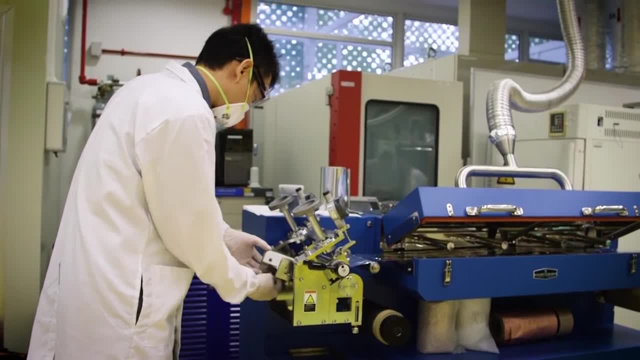 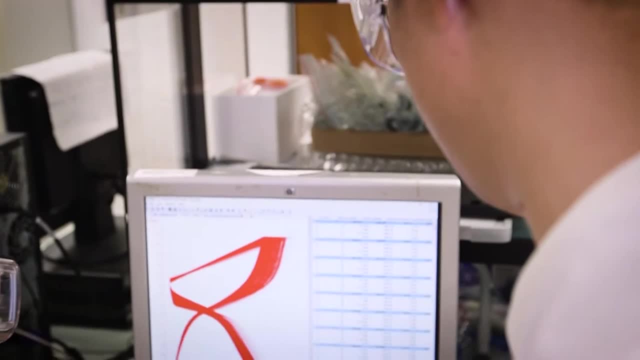 and companies work together to come up with real world solutions. We are looking at how to make batteries safer. We are looking at how do we pack more energy and more power into batteries, And all of this is possible because of the materials that go in as anode. 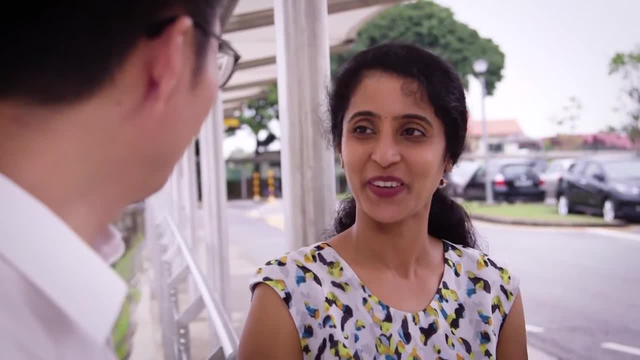 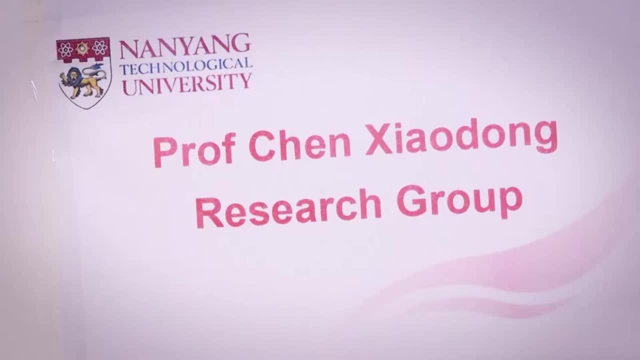 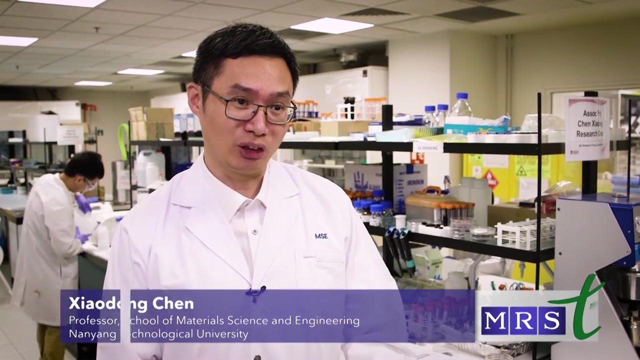 and cathode, And we have a lot of research ongoing on these two areas in the School of Material Science and Engineering. This is a lab for the material synthesis, So once every time we have a new idea to synthesize new materials. this is the place we must have it and give it a try. Recently, we are 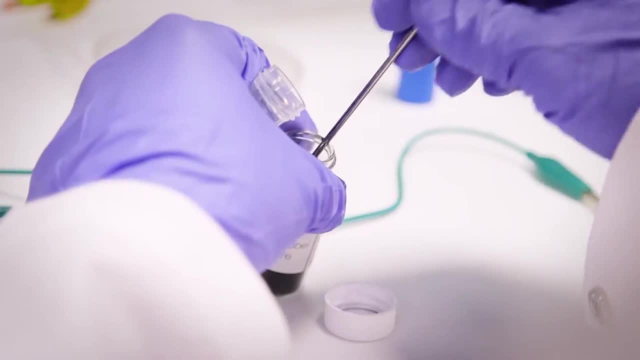 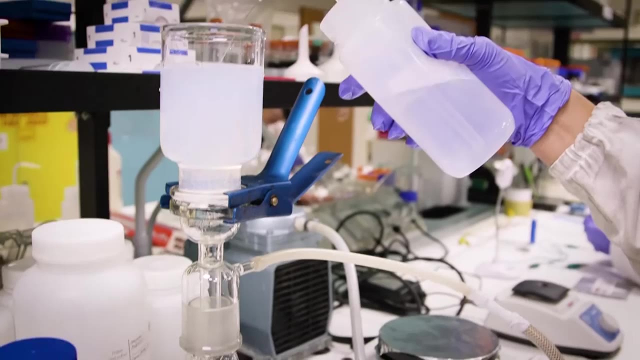 more interested in this kind of far charging nanomaterials, especially based on TR2 materials, which is earth abundant materials. Normally, people synthesize the TR2 materials based on hydrosomal materials, but what we are doing is we add mechanical stirring. This can make new type. 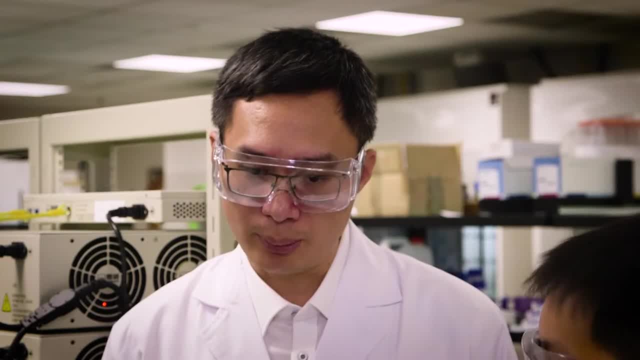 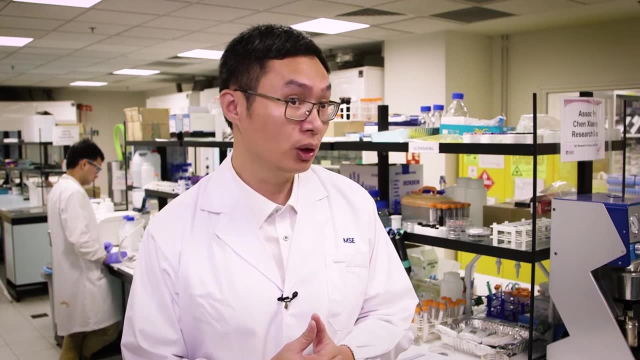 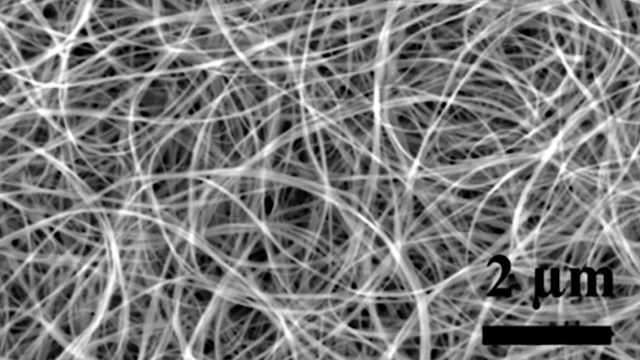 of TR2-based materials. Scanning electron microscope can use to characterize the dimensions of the materials. We also use other kinds of methods, for example X-ray diffraction, which is a method that can tell you the phase. Ultra nanotubes materials can go 30 up to 100 micrometers. 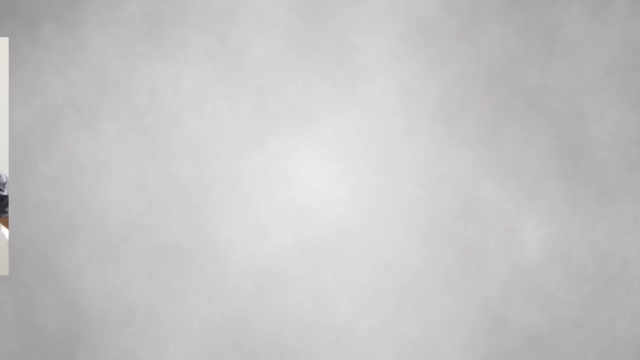 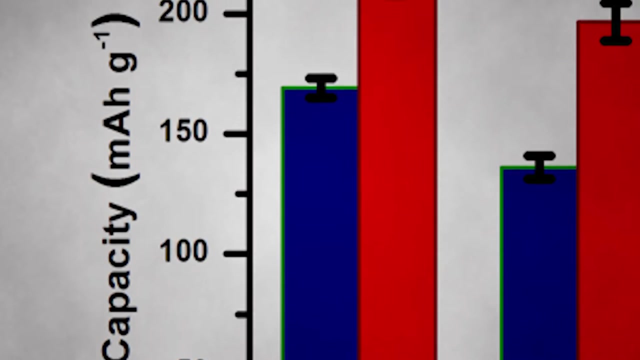 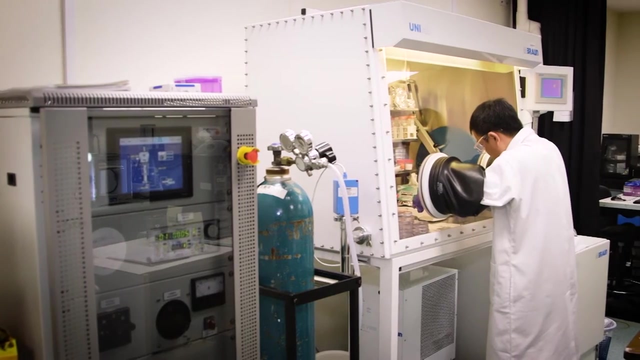 but diameter is only about 10 to 100 nanometers. Because this ultra nanotubes, we don't need too much binder For electromaterial fabrication. this is also the reason why our electromaterials have such a performance in this kind of fast charging and also long life cycle. In the lab we normally 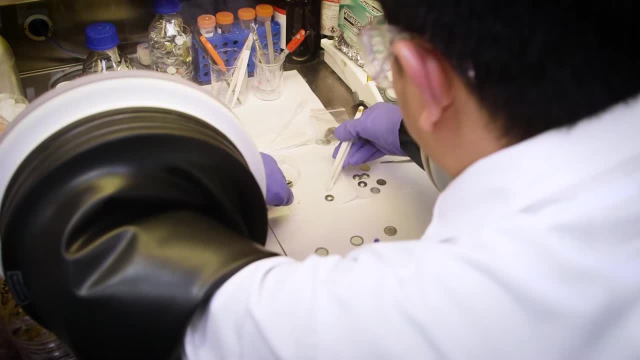 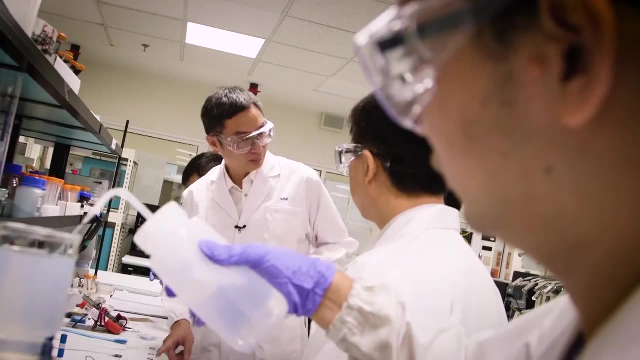 assemble this kind of coin cells. It's very small scale battery. Less than about 5 minutes we can charge it for 70 percent. This is a really important application for this kind of daily use in consumer electronics. Of course coin cell is kind of a demonstration, but 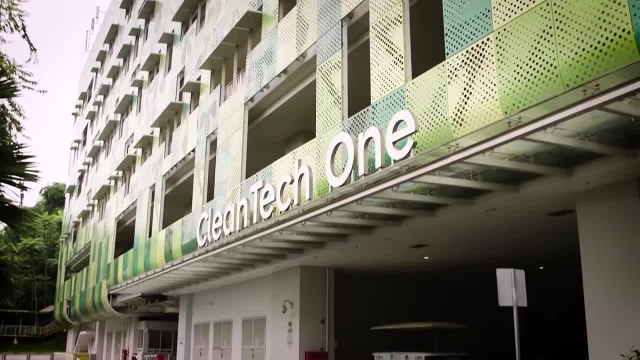 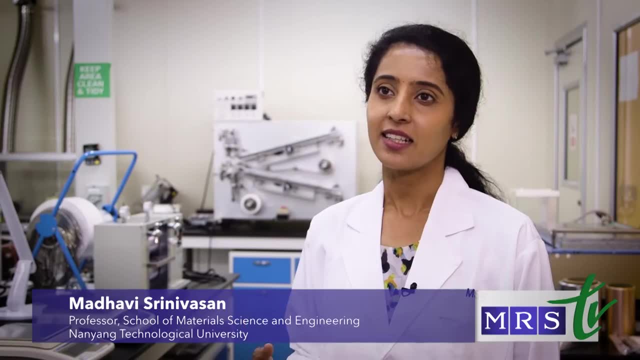 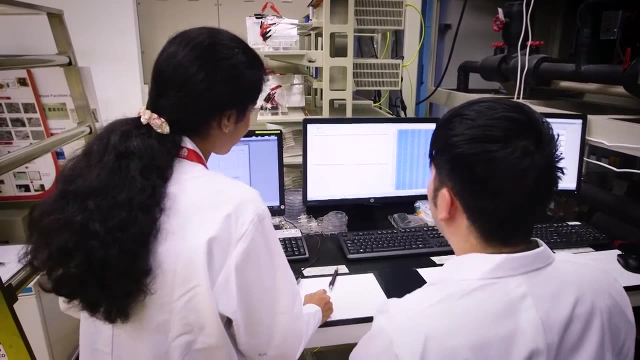 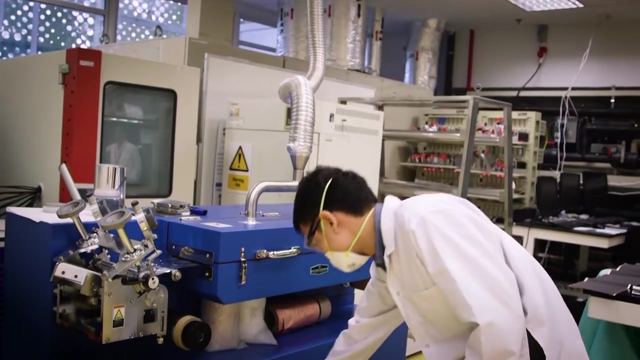 for daily application. we need to scale up. This is a dry room facility for making batteries, and this provides as a bridge between the lab and the industries. The actual performance of this material needs to be tested in a large, real full cell battery before it can be commercialized. TiO2 material needs to be combined with a 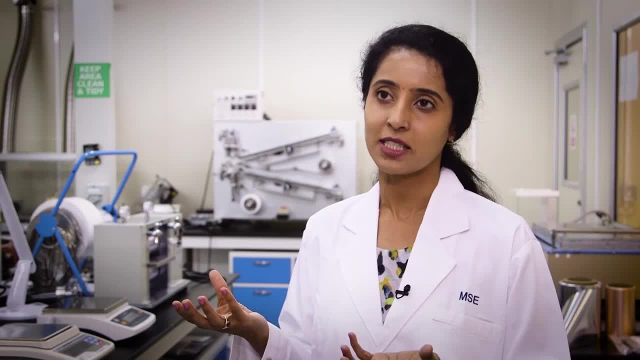 suitable cathode. so we are analyzing a suitable cathode material that can be combined. We will scale up this material and do a test. This is a dry room facility for making batteries and this provides as a bridge between the lab and the industries. TiO2 material also gives us a better capability of proving battery. 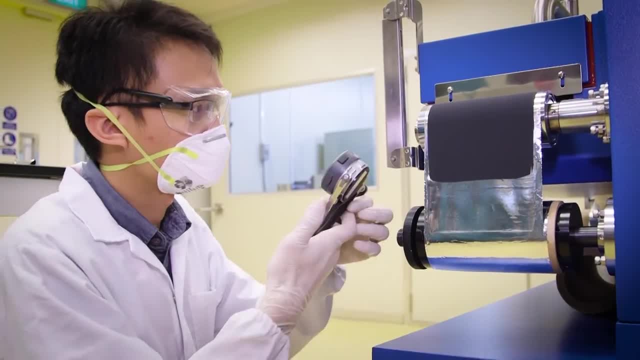 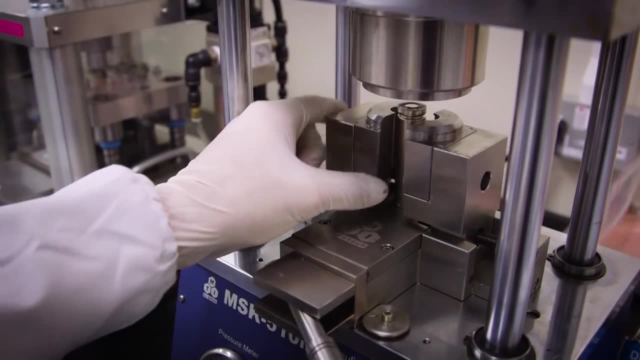 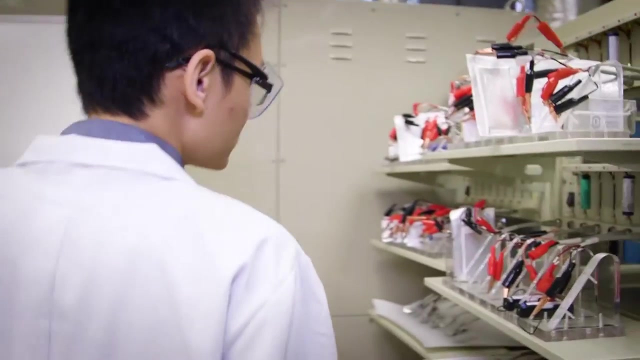 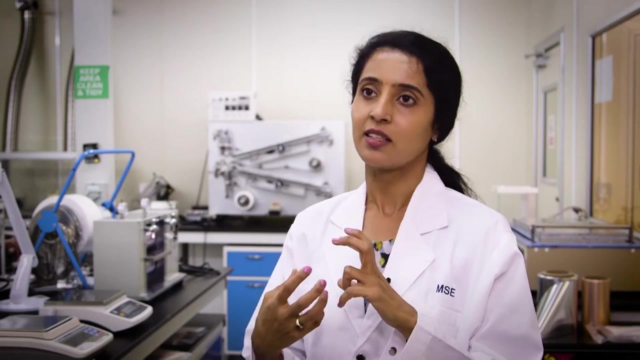 efficiency and it is capable of handling many different 231-肯 T giornal 대박. We keep the batteries in there and we re-attach them to the leading battery and put them into the cell's battery stored and, in terms of longevity. 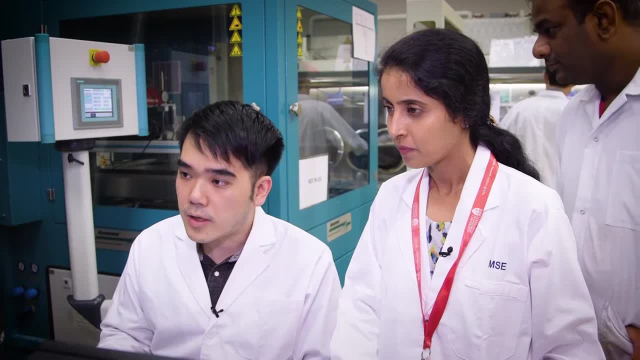 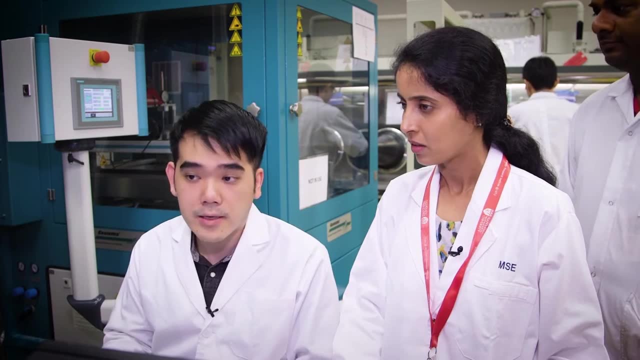 How much is the capacity we are getting for this battery? For this configuration? we are getting about 1,500 mAh. It's been running for about 500 cycles and it is stable. It's about 95% cycle retention. The batteries here have proven very, very effective so far. 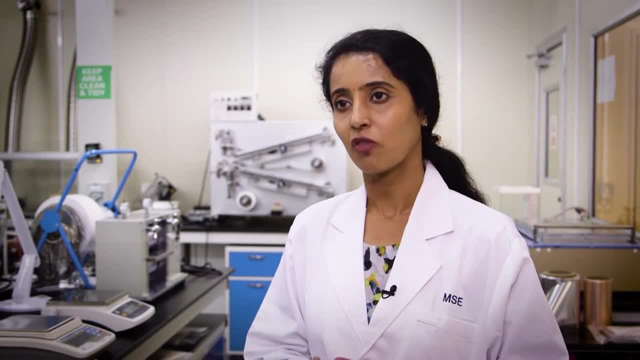 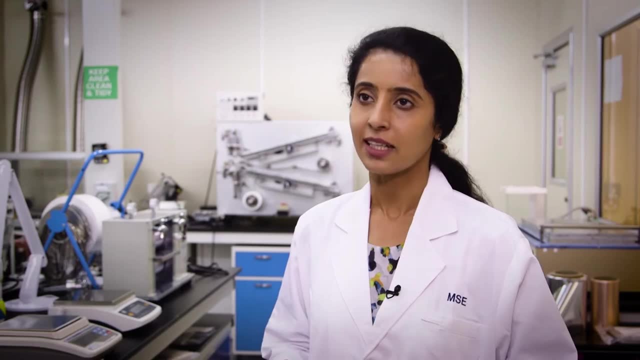 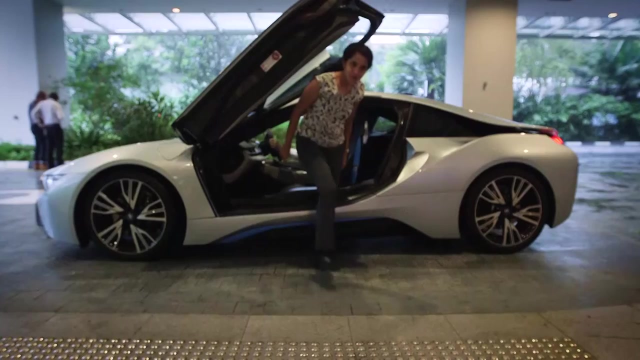 The TiO2 material can enable charging of our battery within minutes rather than within hours, And we have other research going on on other new materials, including electrolytes, The next generation of lithium-ion batteries that will be coming out. NTU MSE has a lot of collaborations with a variety of industries. 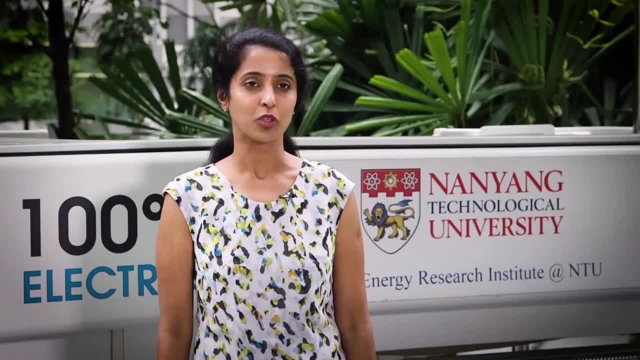 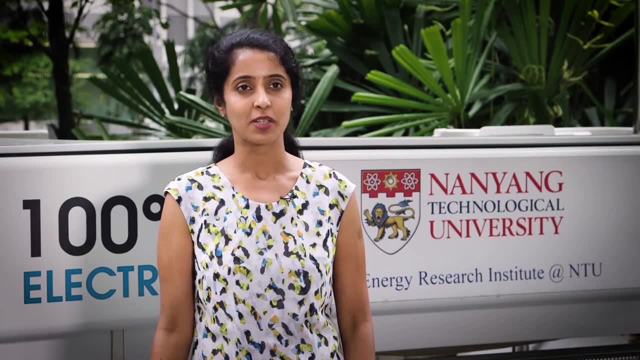 such as BMW, Rolls-Royce, 3M, Procter & Gamble and many more industries, in a variety of materials, starting from biomaterials to battery materials to polymeric materials. The self-driving car behind me is from Navia. 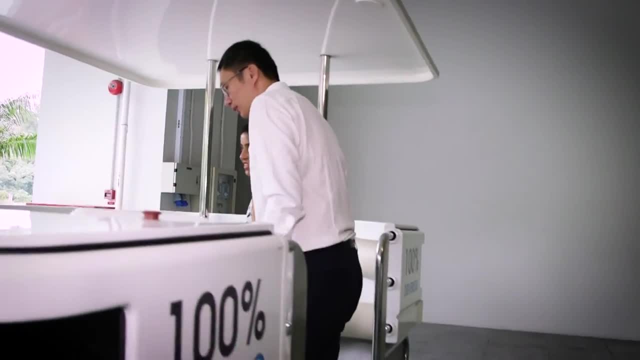 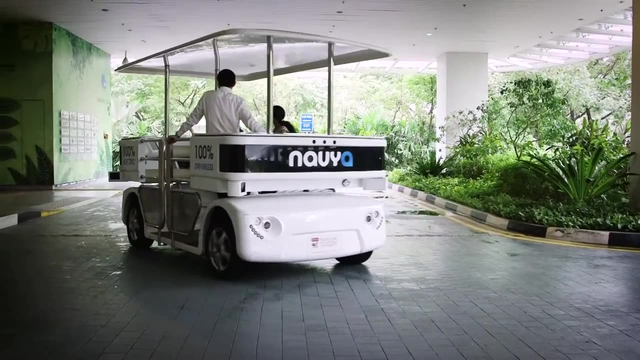 What we are working at NTU MSE is advanced materials which can actually increase the driving range- literally double this driving range- and also reduce this charging time to a few minutes is what we are actually aiming at. The next step in research is really to look at materials. 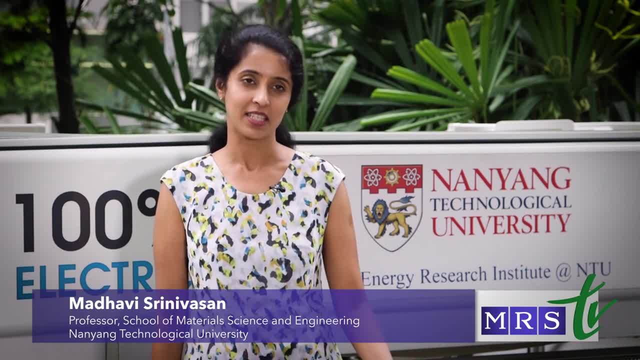 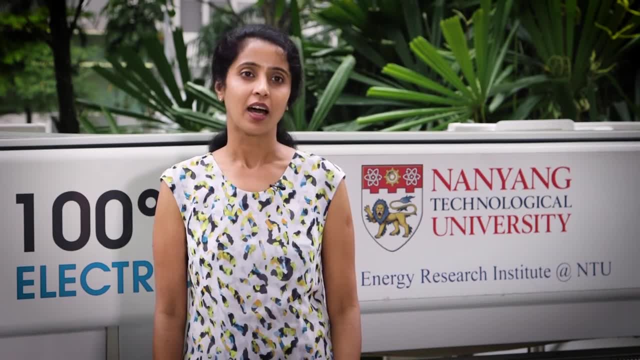 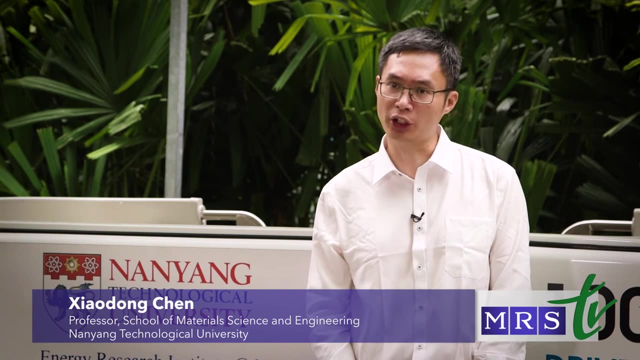 which can store five to ten times the energy than the present day materials. to also enhance the cycle stability so that the battery can last for 10 or 20 years. Last but not the least is to look at the safety aspect of the battery. It potentially allows applications for consumer electronics.